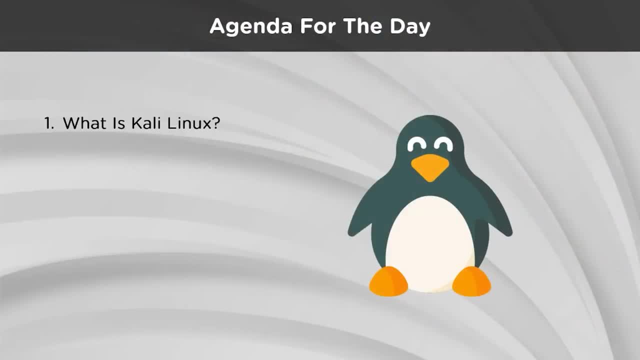 We start by learning about Kali Linux and a basic explanation of its purpose. We take a look at the history of Kali Linux, from the story of its origin to its current day exploits. Next, we learn a few distinct features of Kali that make it an attractive choice for penetration testers worldwide. Finally, we 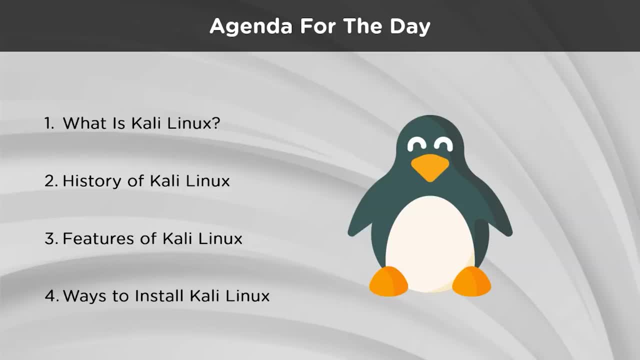 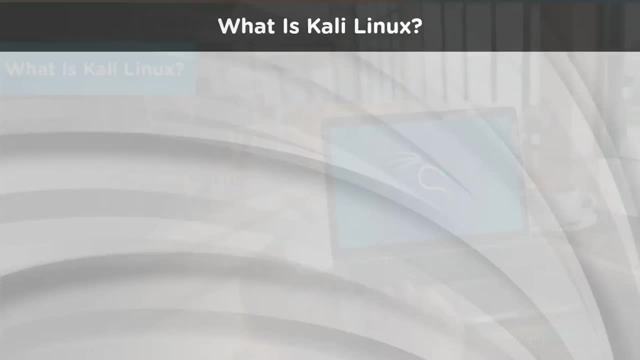 take a look at the multiple ways we can install Kali Linux to start our journey in the world of penetration testing. Let's start by learning about Kali Linux in general. Kali Linux, formerly known as Backtrack Linux, is an open-source Linux distribution aimed 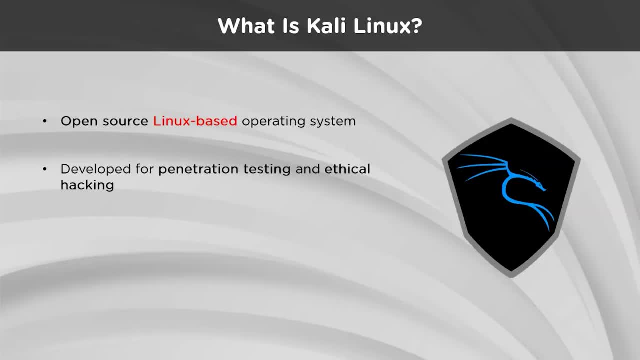 at advanced penetration testing and security auditing. It contains several hundred tools that are targeted towards various information security tasks, such as penetration testing, security research, computer forensics and reverse engineering. Kali Linux is a multiple platform solution accessible and freely available to information security professionals and 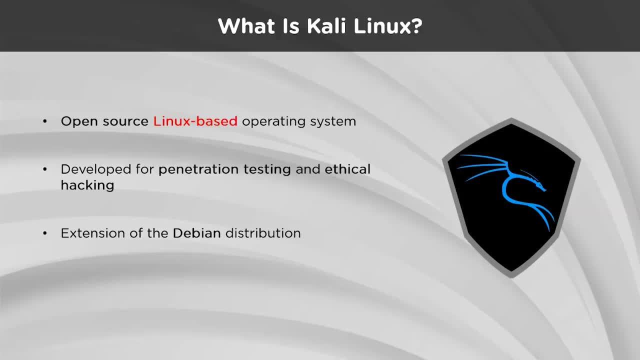 hobbyists. Among all the Linux distributions, Kali Linux takes its roots from the Debian operating system. Debian has been a highly dependable and stable distribution for many years, providing a similarly strong foundation for the Debian operating system. Debian has been a highly dependable and stable distribution for many years, providing a similarly strong 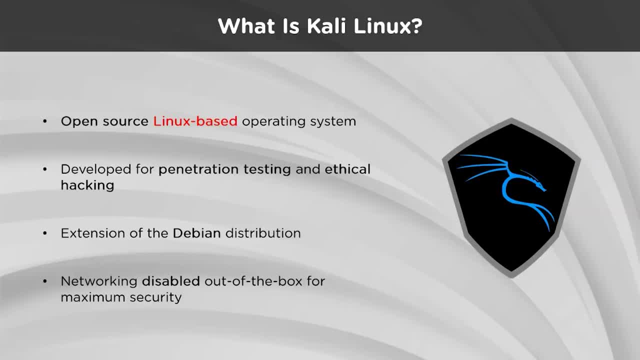 foundation for the Kali desktop. While the operating system is capable of practically modifying every single part of our installation, the networking components of Kali become disabled by default. This is done to prevent any external factors from affecting the installation procedure which may pose a risk in critical environments. Apart from boosting security, it allows a 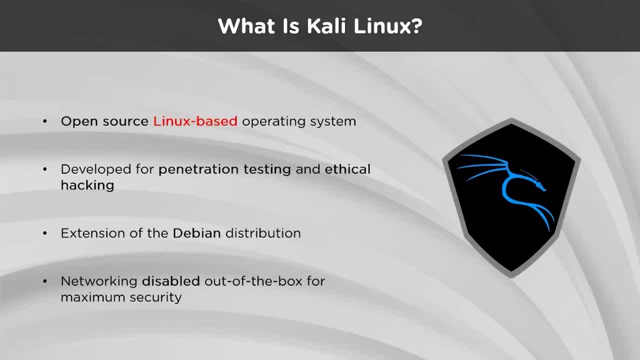 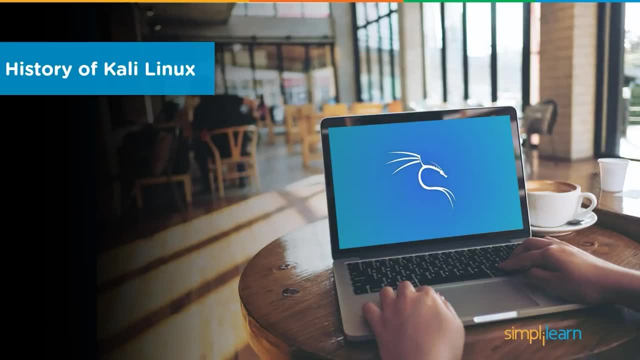 deeper element of control to the most enthusiastic of users. The data has been shamefully used to control Kali, but not to provide information to our the first day. How did it come into existence? Let's take a look at some of its history. 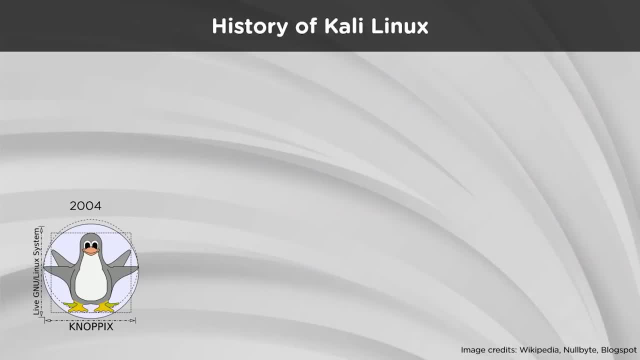 Kali Linux is based on years of knowledge and experience in building, penetration, testing and operating systems. During all these project lifelines, there have been only a few different developers, as the team has always been small. The first project was called Wopex, which stands: 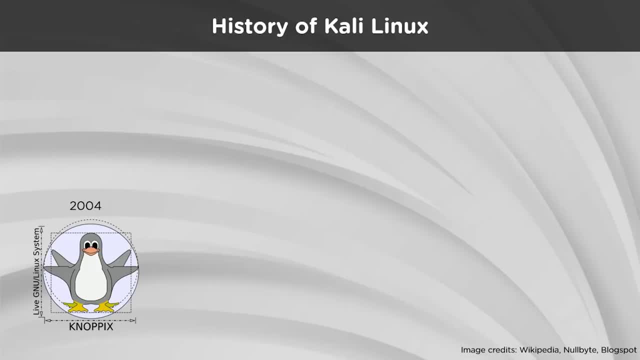 for White Hat Knopex. As can be inferred from the name, it was based on the Knopex operating system as its underlying OS, Wopex, had releases ranging from version 2.0 to 2.7.. This made way for the 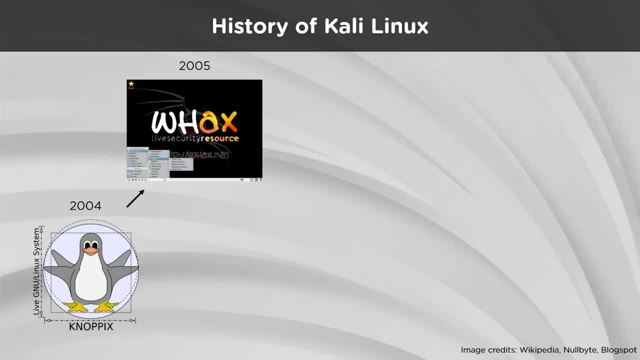 next project, which was known as Wax or the long hand being White Hat Slacks. The name change was because the base OS was changed from Knopex to Slacks. Wax started at version 3 as a nod it carrying on from Wopex, There was a similar OS being produced at the same time. 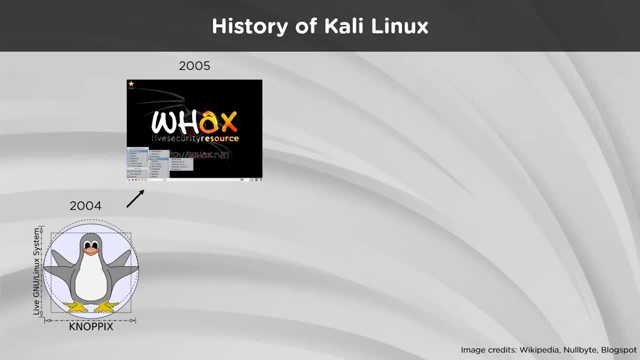 Auditor Security Collection often being shorter to just Auditor, which was once again using Knopex. The same time, Auditor Security Collection was being shorter to just Auditor, which was once again using Knopex. Its efforts were combined with Wax to produce Backtrack. Backtrack was based on Slackware. 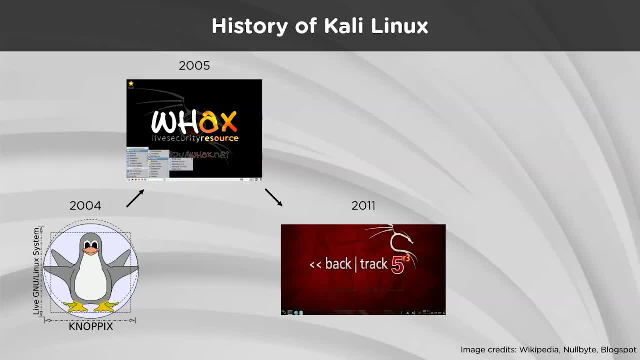 from version 1 to version 3, but switched to Ubuntu later on, with version 4 to version 5.. Using the experience gained from all of this, Kali Linux came after Backtrack in 2013.. Kali started off using Debian stable as the engine under the hood before moving to 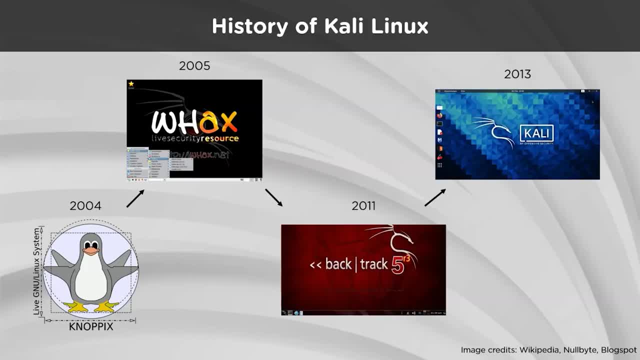 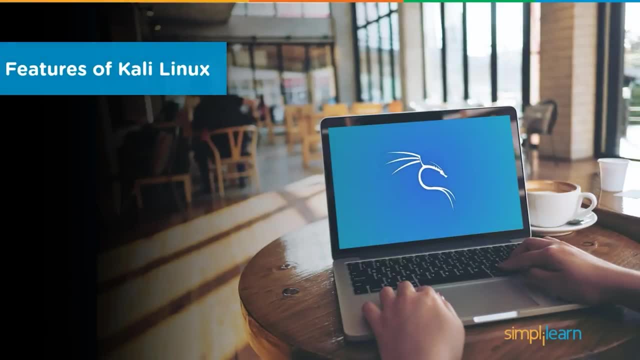 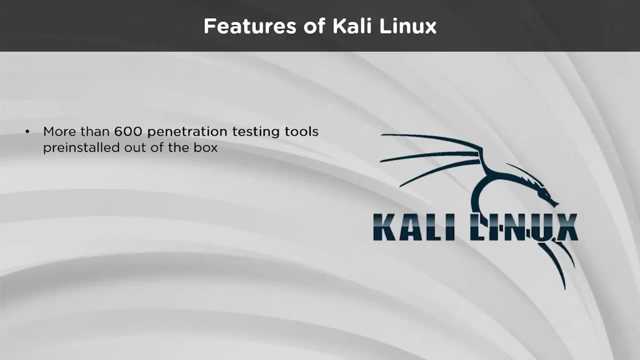 Debian testing when Kali Linux became a rolling operating system. Now that we understand the history and the purpose of Kali Linux, let us learn a little more about its distinct features. The latest version of Kali comes with more than 600 penetration tools pre-installed. 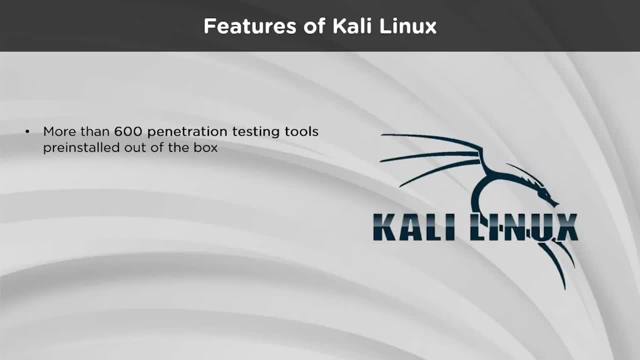 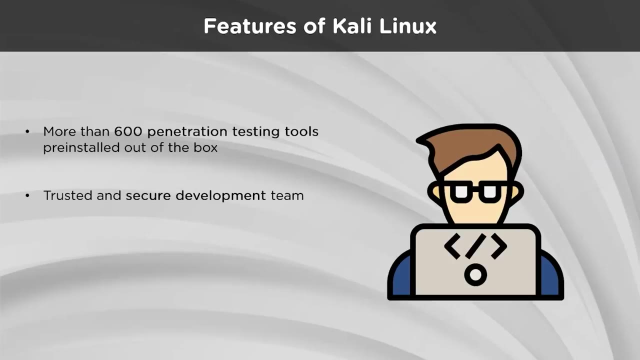 After reviewing every tool that was included in Backtrack, developers have eliminated a great number of tools that either simply did not work or which duplicated other tools that provided the same or similar functionality. The Kali Linux team is made up of a small group of individuals who are the only ones trusted to commit packages and interact with. 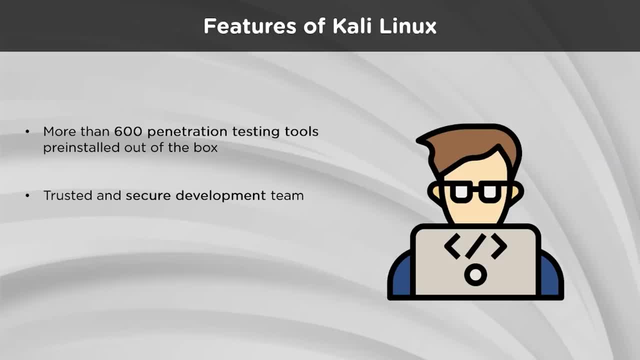 the repositories, all of which is done using multiple secure protocols. Restricting access of critical code bases to external assets greatly reduces the risk of source contamination, which can cause Kali Linux users worldwide a great deal of damage as a direct victim of cybercrime. 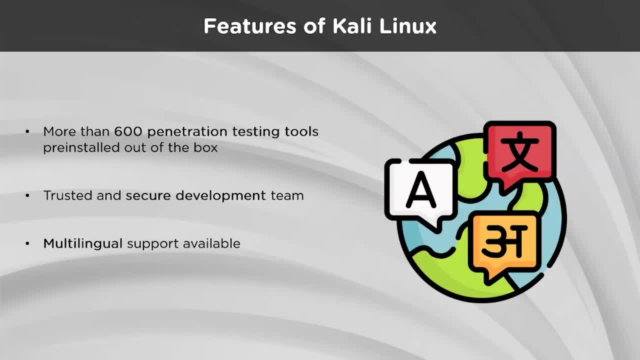 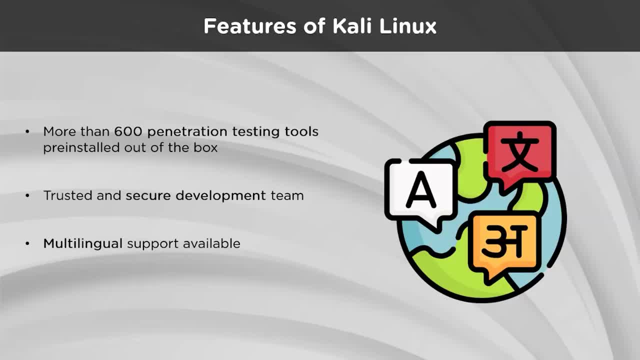 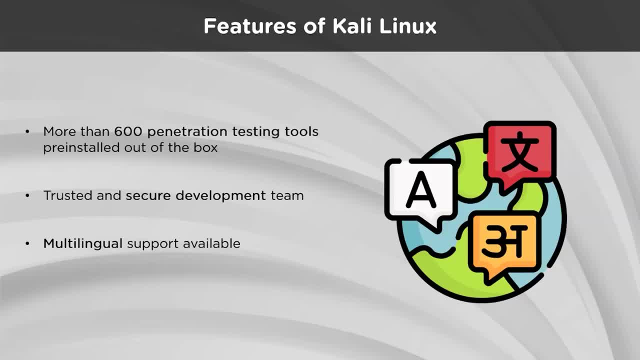 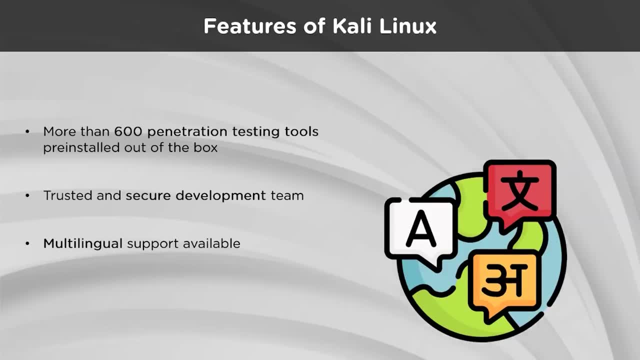 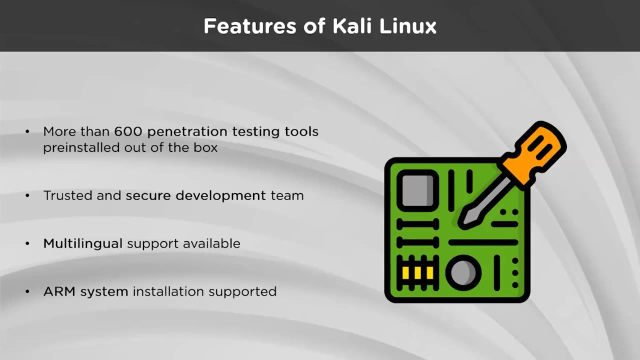 job. The more comfortable a user feels with the intricacies of the operating system, the easier it is to maintain a stronghold over the configuration and the device in general. Since ARM-based single-board systems like the Raspberry Pi are becoming more and more prevalent and inexpensive, the development team knew that Kali's ARM support would need to be as robust as 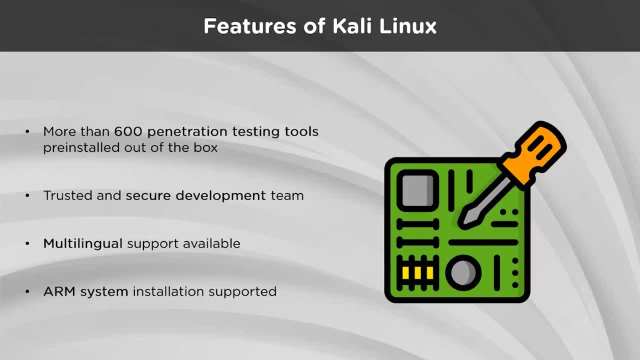 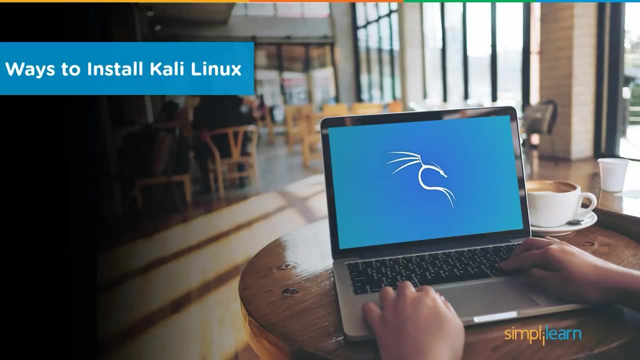 they could manage with the help of a single-board system like the Raspberry Pi. Kali Linux is available on a wide range of ARM devices and has ARM repositories integrated with the mainline distributions, so the tools for ARM are updated in conjunction with the rest of the distribution. All this information is necessary for users to determine. 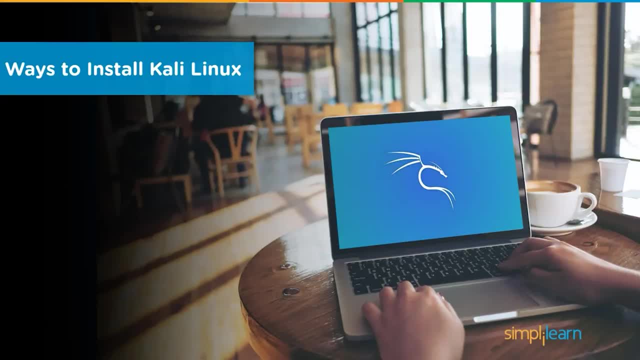 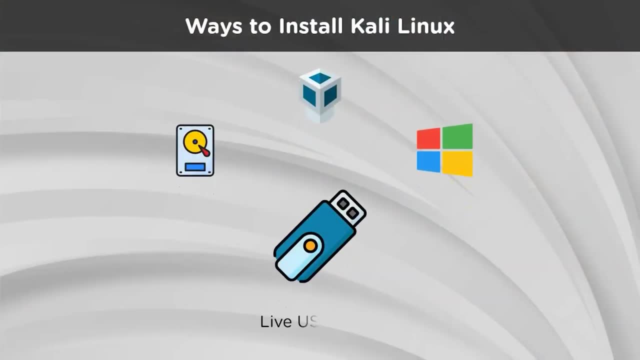 if Kali Linux is the correct choice for them. If it is, what are the ways that they can go forward with this installation and start their penetration testing journey? The first way to use Kali Linux is by launching the distribution in the live USB mode. This can be achieved by downloading the 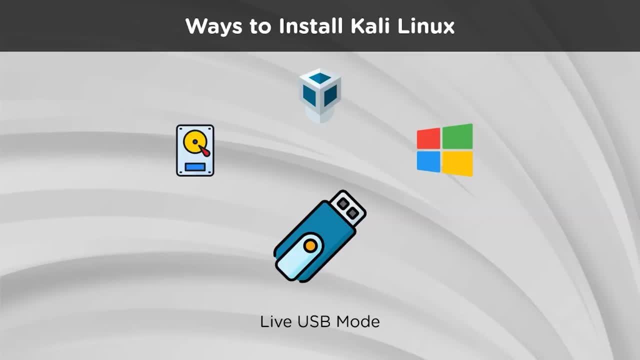 installer image file or the ISO file from the Kali Linux website and flashing it to a USB drive with a capacity of at least 8 GB. Some people don't need to save their data permanently and a live USB is the perfect solution for such cases. After the ISO image is flashed, the thumb drive can be. 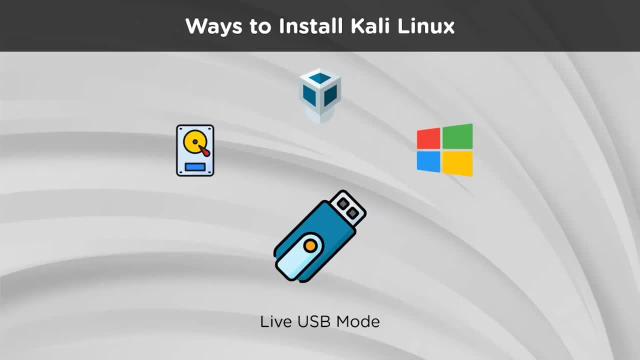 used to boot a fully working installation of the operating system, with the caveat that any changes mode are not written permanently. Some cases allow persistent usage in live USBs, but those require further configuration than normal situations. But what if the user wants to store? 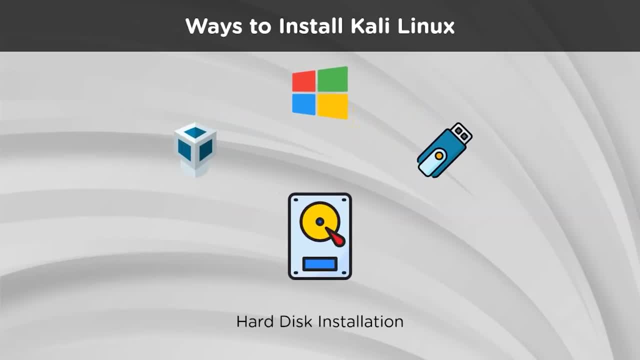 data permanently in the installed OS. The best and the most reliable way to ensure this is the full-fledged hard disk installation. This will ensure the complete usage of the system's hardware capabilities and will take into account the updates and the configurations being made to the. 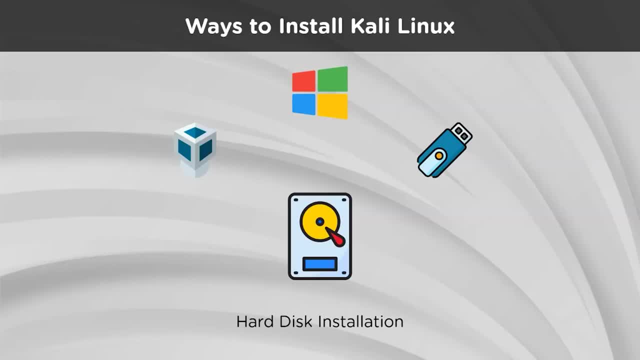 OS. This method is supposed to override any pre-existing operating system installed on the computer, be it Windows or any other variant of Linux. The next alternative route for installing Kali Linux would be to use virtualization software such as VMware or VirtualBox. The software will be installed as a separate application on an